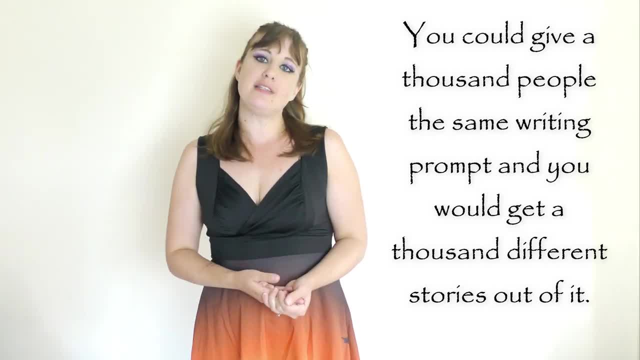 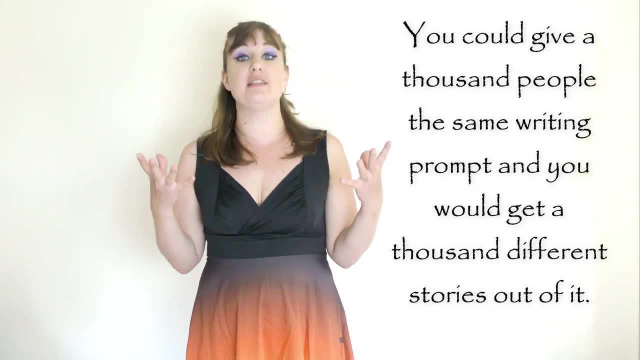 different ideas, a thousand different stories, because we all see the, the writing prompt that we are given and we come up with different ways to write it. So I'm going to talk to you about that and I'm going to give you a little bit of an example of what that is, So you can see that. 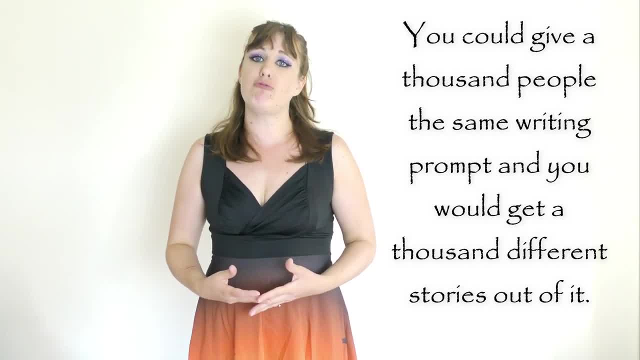 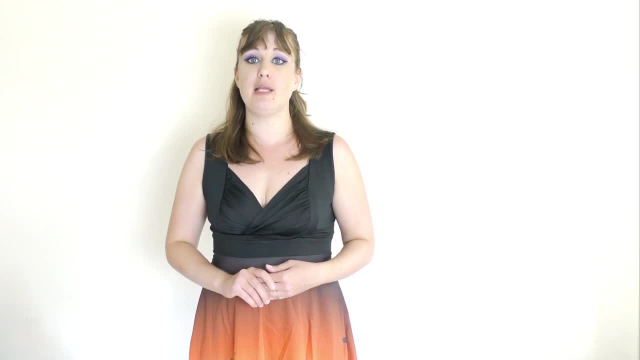 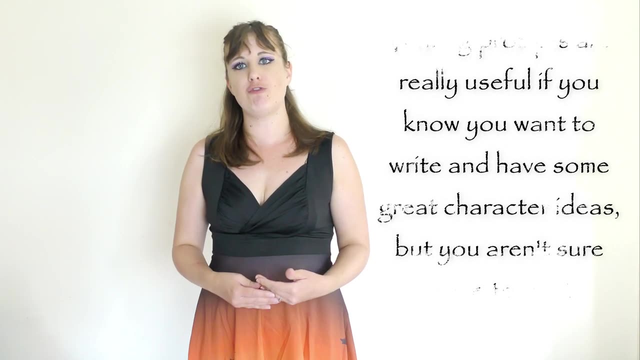 there are different ways of addressing it, different thoughts. it inspires us in different ways and you will create from that little prompt. you will create different characters, different scenarios, different back story, different conflicts. everything will be completely unique. you're just using one tiny starting point, so writing prompts are fantastic, especially if you're struggling for 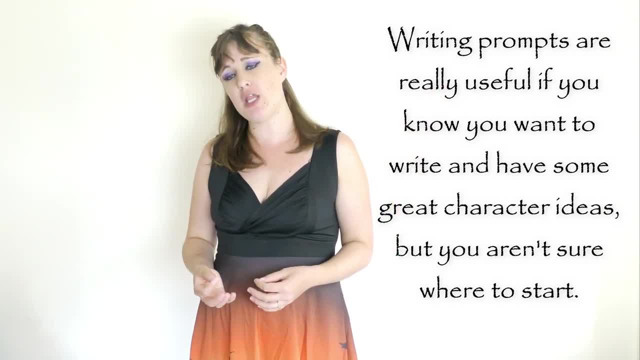 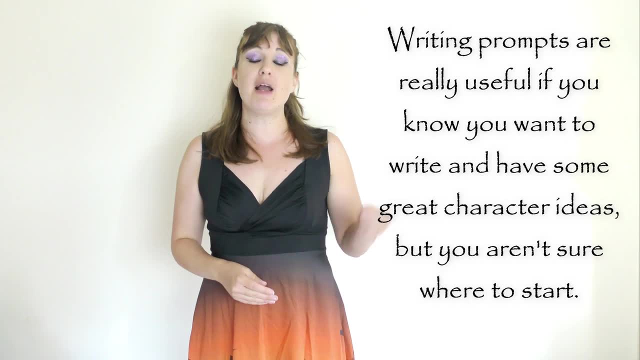 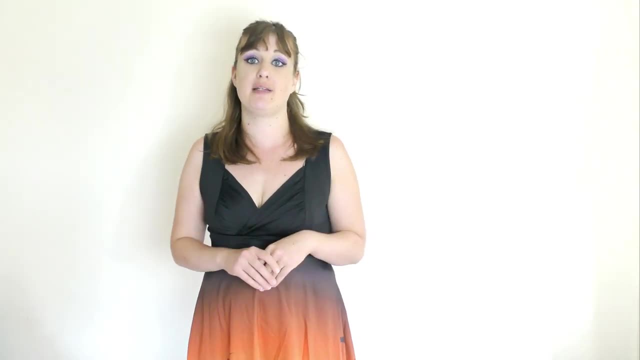 an idea and you know you want to write and you have really good characters and things in your head, but you're not sure where to start with. You're just throwing it. it's like lightning. you have all these ideas come out from it. so writing prompts are fantastic and you can find them. they're all over Twitter, Instagram, thousands and thousands on Pinterest. fantastic, highly recommend it. 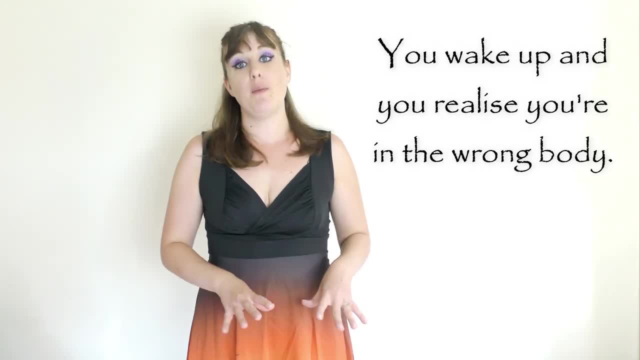 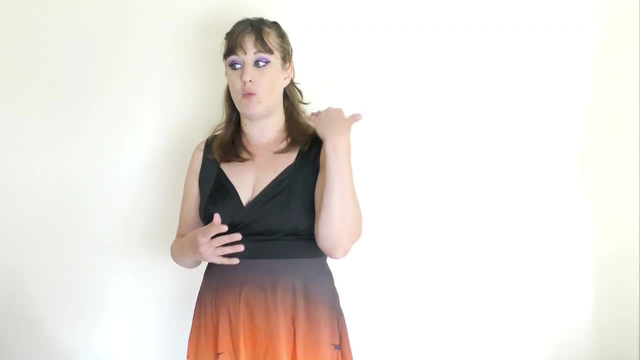 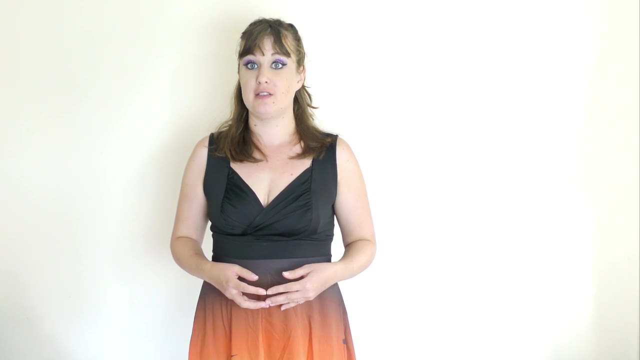 So the writing prompt I'm going to talk about today is: you wake up and you realize that you are in the wrong body. So the question I was given was: what would you do, which is what I'm going to use for the writing prompt. So, first thing, you do. there are multiple things you might do. first, 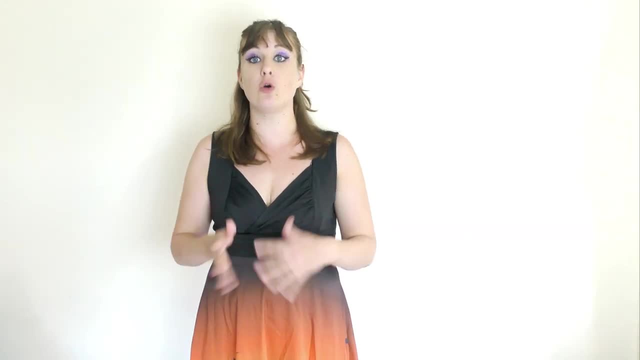 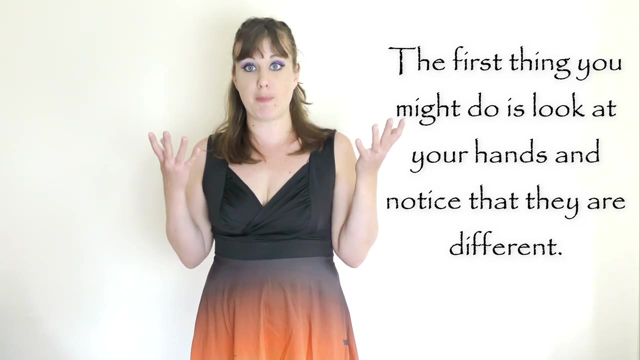 So this is my point. you will all come up with different things, so I'll just talk through a few of them. First thing you might do is notice. notice, I mean, if you think about it, wake up. you aren't immediately looking down at yourself, you aren't looking at yourself in a mirror, but you do look at your. 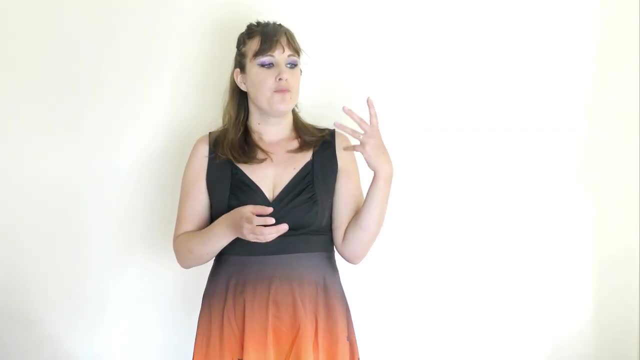 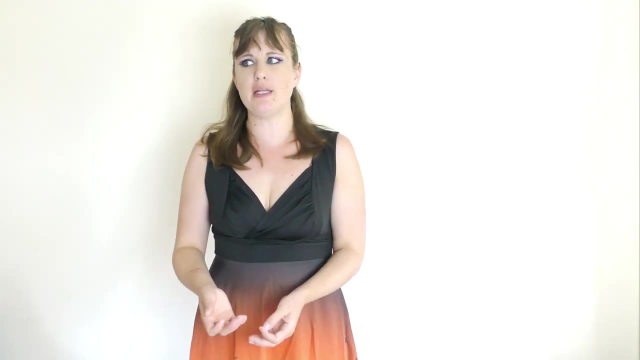 hands so you pick up your phone to see what time it is, or you just you wake up and you're like that. you might notice that your hands are wrong, but you might not immediately realize they're wrong. you might just be a bit foggy eyed and confused. 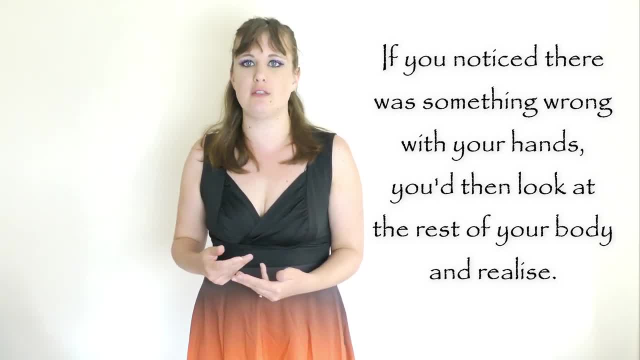 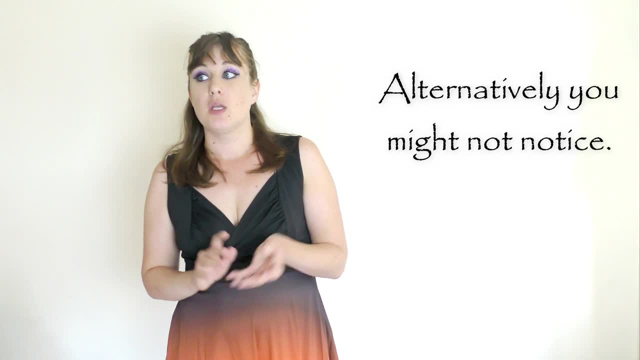 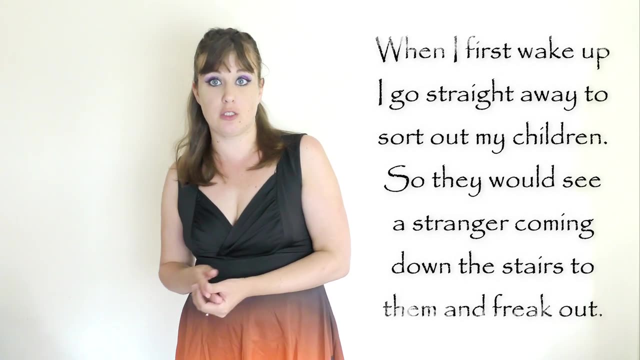 But if you notice there's something wrong with your hands, then you might start to look at the rest of you and then you'd realize. Alternatively, you might not notice at all, you might not realize, you might wake up and just get up, like for me, for instance. when I first wake up I usually have to go sort out my children. 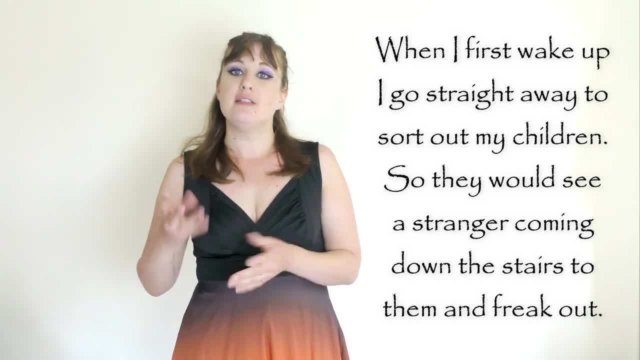 because one of them has been like: mommy, I need the toilet or mommy, I want my breakfast. So we get up, I head downstairs. but then, if that happened, if one of my children woke me up, if I went downstairs and I'm somebody else and a stranger came walking down the stairs and the other one just woke me up and said: 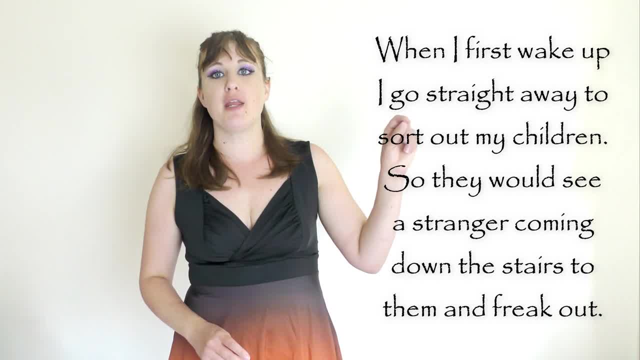 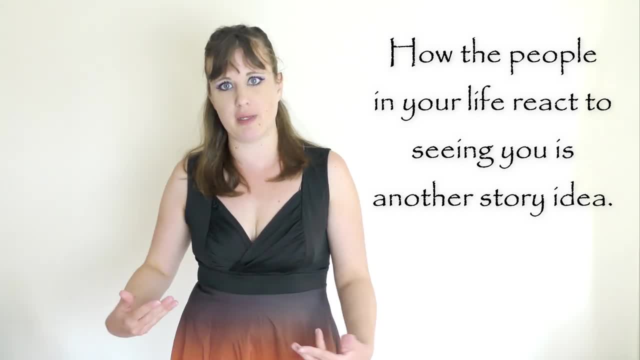 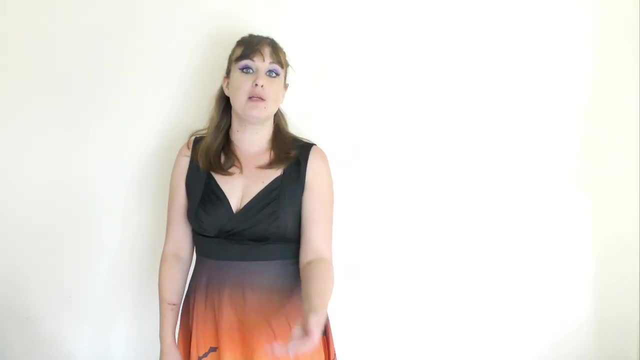 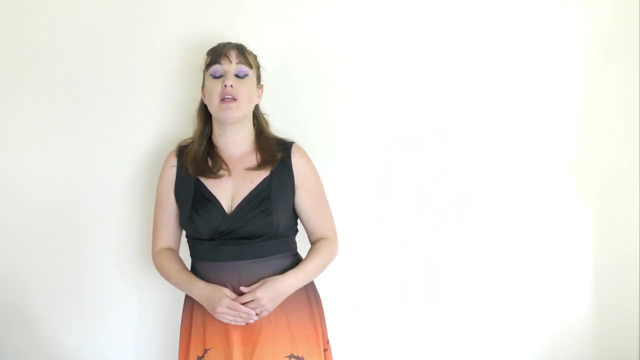 you go downstairs, you make your coffee, maybe you go to the toilet, you look in the bathroom mirror and see somebody different staring back at you, then of course, then it's a different freak out, a different panic, because then you're having a different story. so then, when your character or you 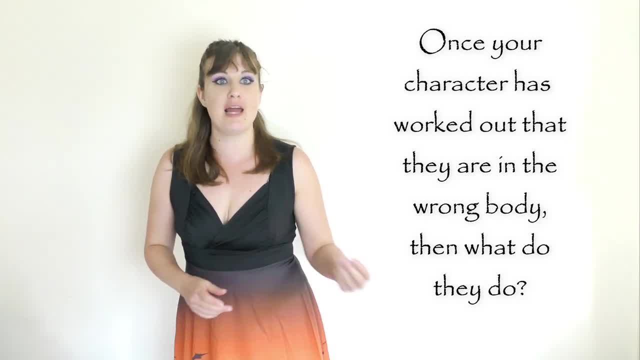 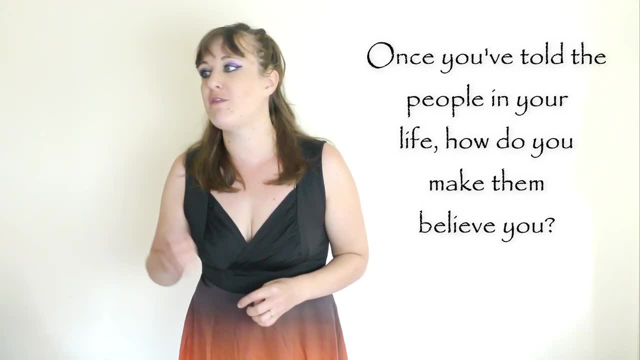 your character has worked out that they are in the wrong body. then what do they do? if they're in a relationship, they have to wake up their partner and tell them. if they're at home with their parents, again they have to tell them. if they have kids. how do they explain to their kids? and 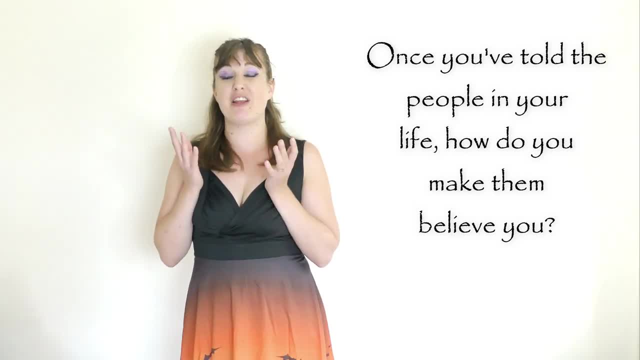 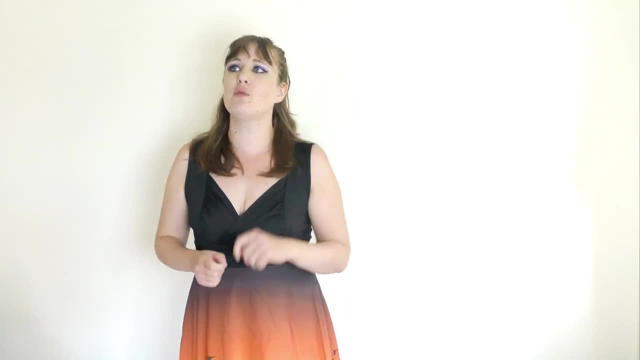 then would they believe them? would they not think that they are just some crazy stranger who's broken into the house and is trying to convince them? so then it's what questions would they ask? how would you prove it was really you? and then you have to work out who did it to you. how did it happen is? 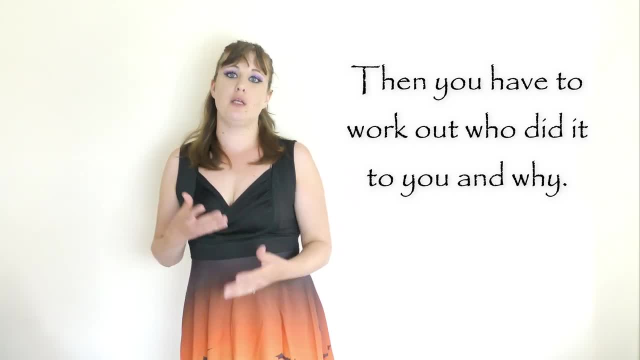 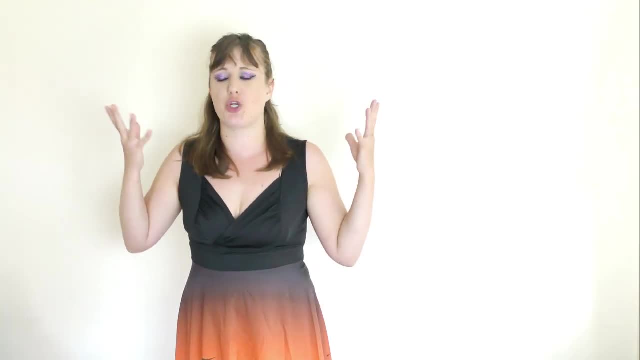 it some kind of freaky friday thing where you have to sort of work out who did it to you and learn the truth by a certain time so that you can switch back like: is it a body swap or is like somebody's cursed you and put a spell on you and then you're in the wrong body? is it going to stay? 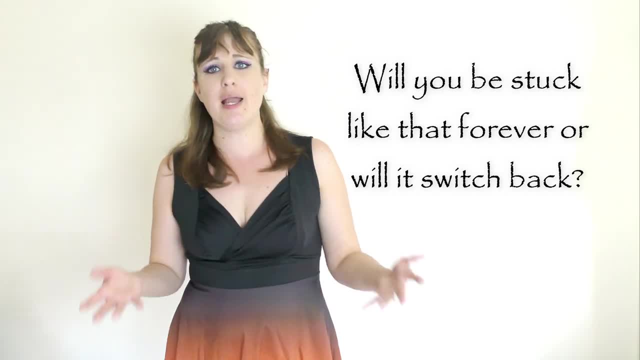 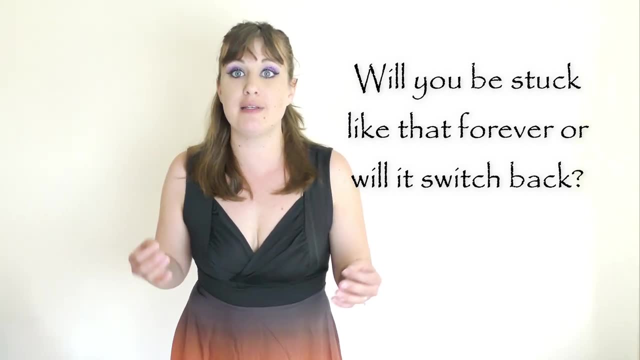 like that forever? do you then have to try and explain to the outside world why your partner is suddenly in a different relationship with a different person? but it's still you. would they believe you? how is it going to affect your whole life that you are suddenly in the wrong body? 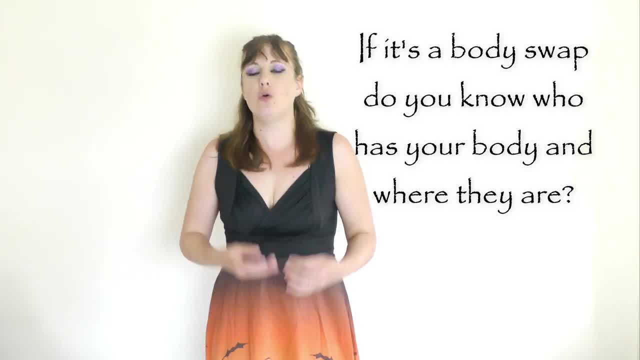 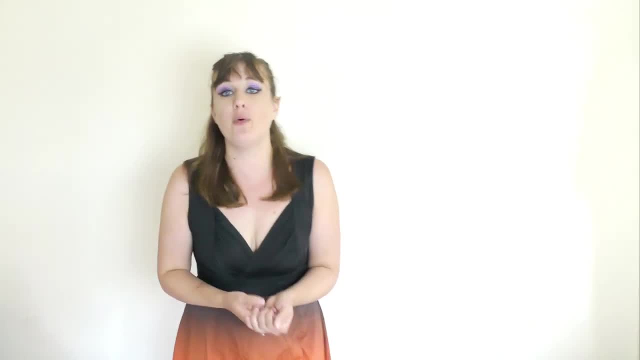 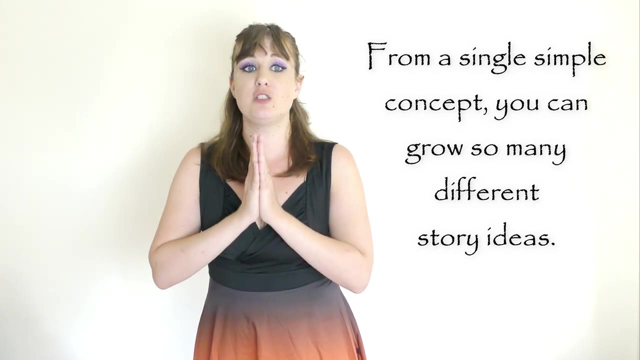 who has your body? do you know if someone has your body? oh, there's so many questions. i love writing prompts- probably tell getting over it excited, but i do. i love writing prompts because that's the point. once you start thinking about a scenario, just a simple little scenario, so many stories can spring from it and yeah, so that's the. 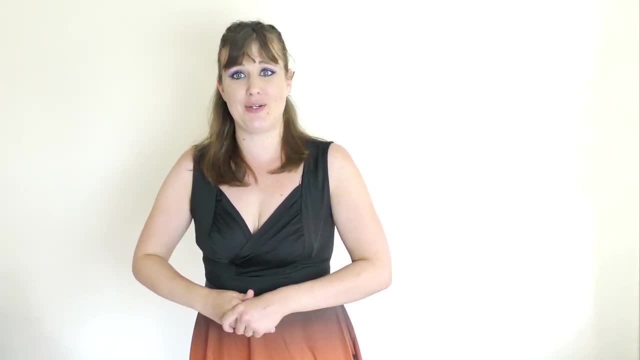 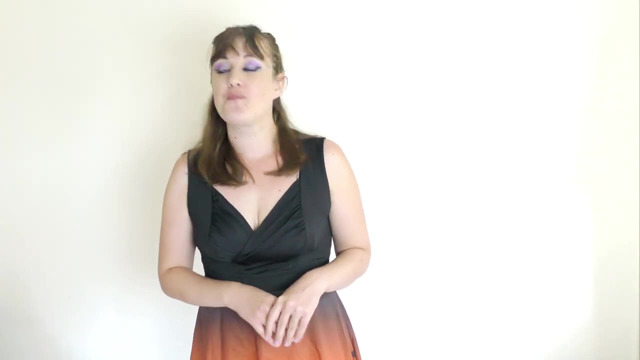 writing prompt thought. so what i would like to deal? and i don't set homework. and i'm not going to set homework. obviously of course i'm not. but what i am going to do is say maybe if a few people who want to do it can do it. and i'm not going to do it and i'm not going to do it and i'm not going. 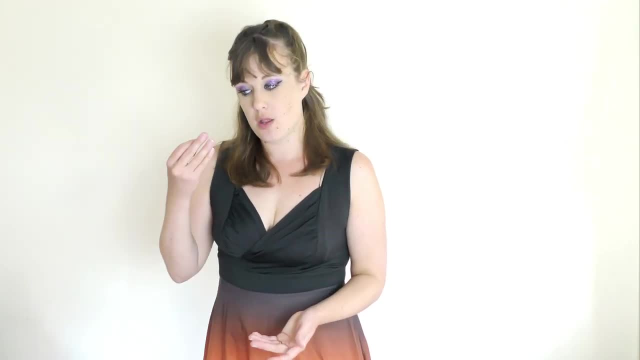 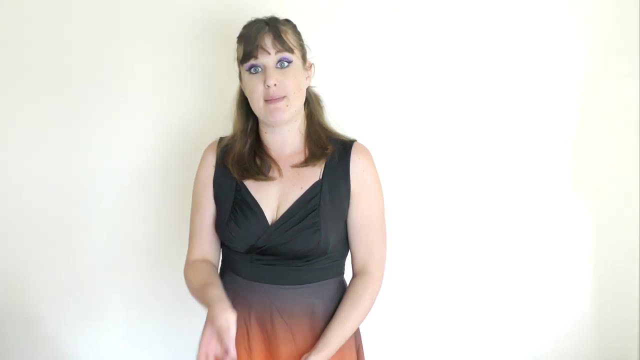 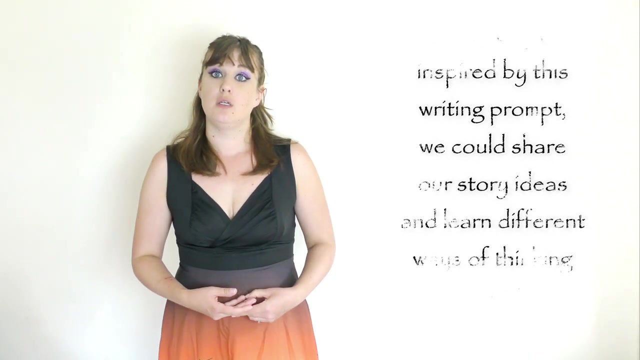 to watch these videos. go away. think about waking up and realizing they're in the wrong body maybe. i mean, there's all sorts of social medias, as well as the youtubes, that we could share those on and we could look, and we could look at how other people have responded to a writing prompt. 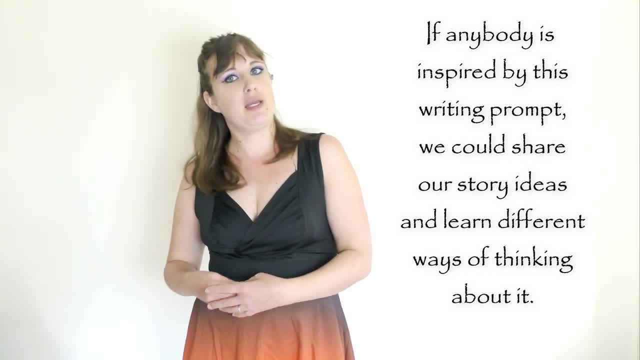 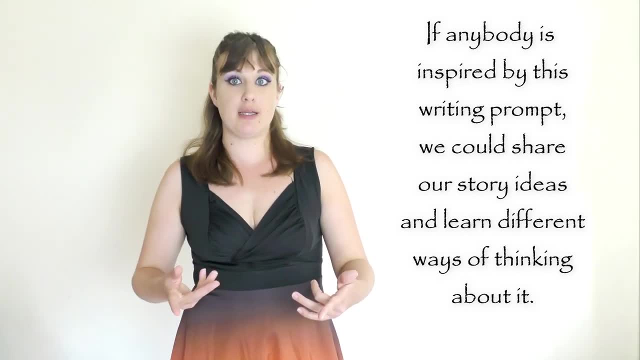 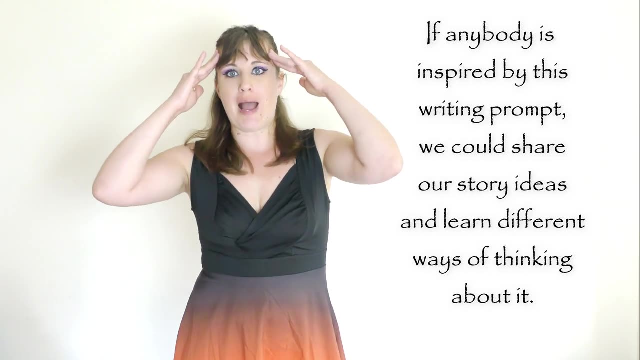 and work out why and what we can learn from it, and maybe explore that a bit, because that would be to me really interesting to see how you guys respond to it, what thoughts come into your head, and i think we can learn a lot from that, because we always follow our thoughts. but if you see, 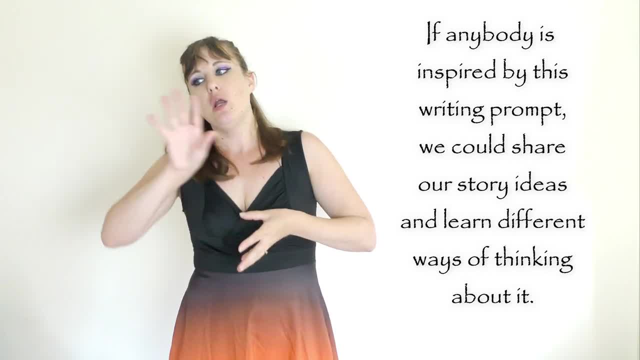 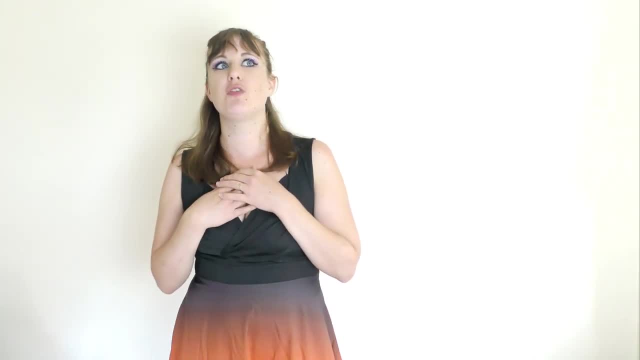 where someone has come from with a writing prompt and how their mind has shut off with it. it can give you new ideas and new ways of thinking, and i think that would be a really interesting thing. of course, you don't have to do it. i'm not going to be checking up on you. 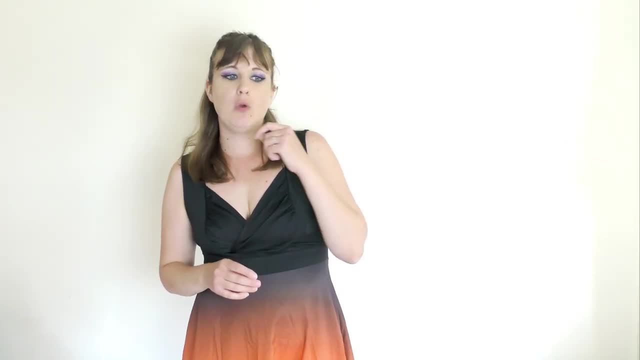 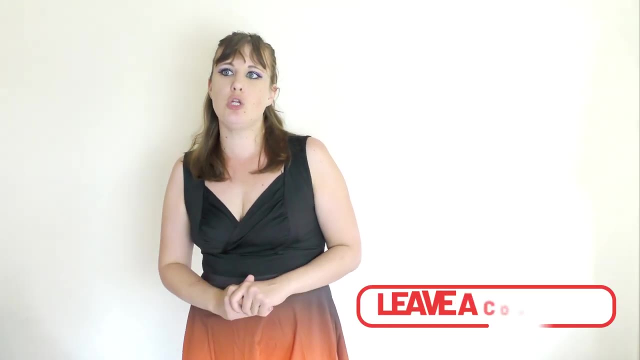 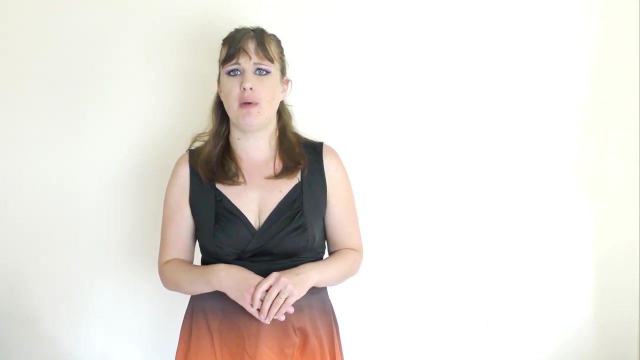 but if you wanted to take part and do that, where would we share it? put me a comment below where you think we should all put these, whether it's here on youtube or somewhere else. um, but i would really like to see what other people come up with, because i think it's a really interesting concept. 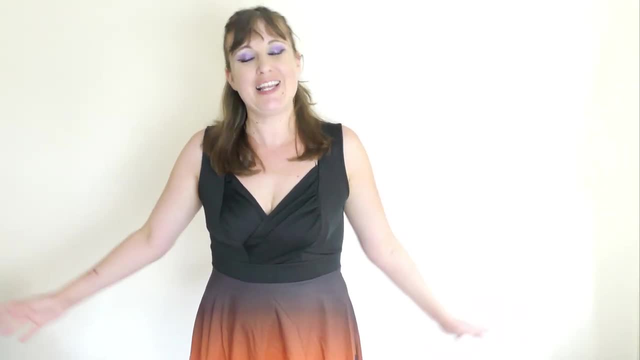 so, yeah, we should all try- as many of us as we want to, obviously and think about what we would do if we woke up when we're in the wrong body. we should all try and think about what we would do if we woke up when we're in the wrong body. 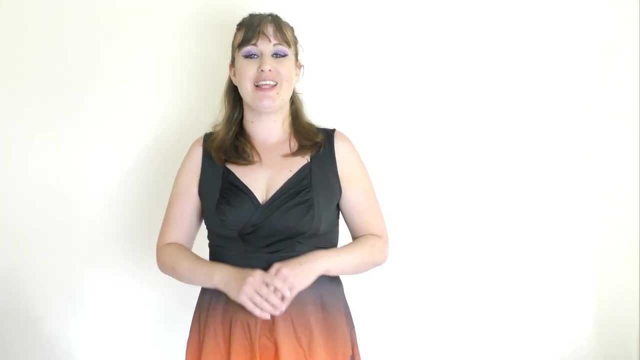 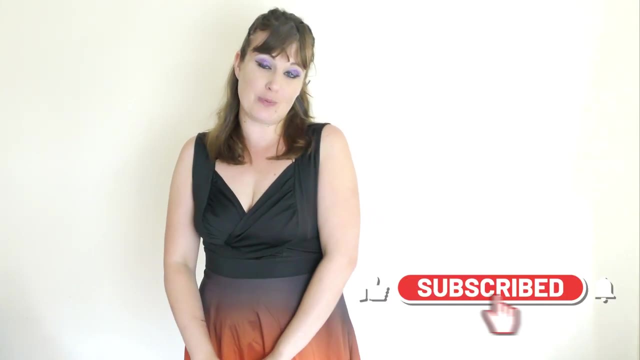 and think of the characters and the scenarios that we would get into, because it's a really interesting writing prompt. so thank you very much for watching. please subscribe to this channel. as i say, monday, wednesday and friday is when i'm putting videos out, normally, unless i'm sick and 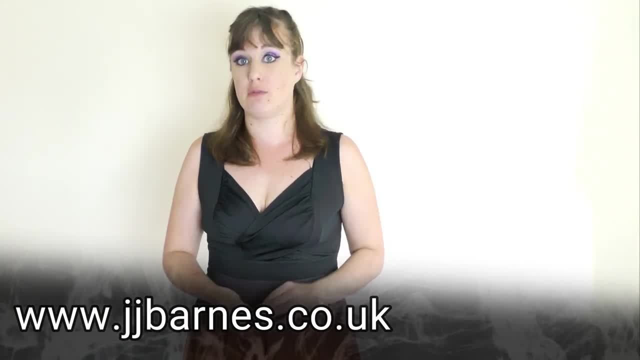 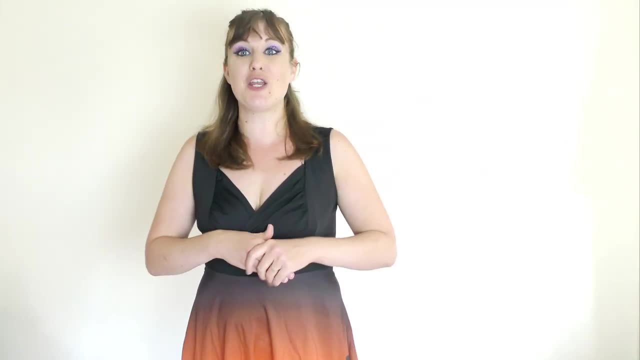 or if you go to my website, jjbarnescouk, over there, you'll find links to all my social media, as well as all the work i'm doing and my books, things like that. so come find me, talk to me and tell me what you think of the writing prompt and if this video is popular and successful and people.